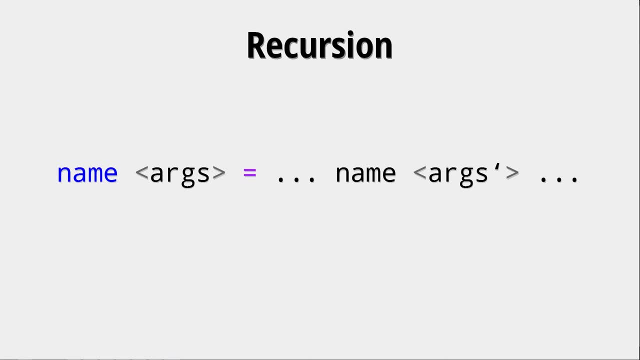 in Haskell There are no loops. So if you want something to loop in a sense you have to use recursion, So a function calling itself with some other arguments, or maybe even the same arguments, even though that wouldn't make much sense. So this is the basic boilerplate of how. 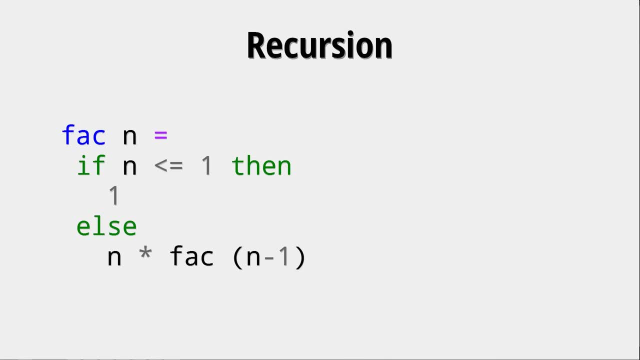 recursion looks like. Let's look at an example, the prime example for recursion, which is the faculty function. Now, in this case, we say that, okay, the faculty of n smaller or equal to one should be one, And otherwise we have this recursive call. we say that the definition. 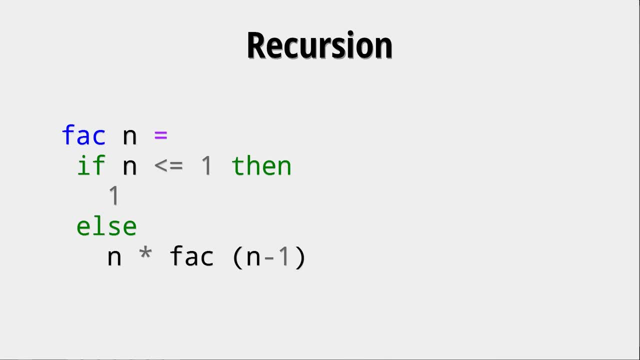 of the faculty of n is n times the faculty of n minus one. That is also the mathematical definition of the faculty. If we look at how the evaluation works, we see it works sort of as expected. the faculty of three is of course three times the faculty of two, and so on and so forth. And 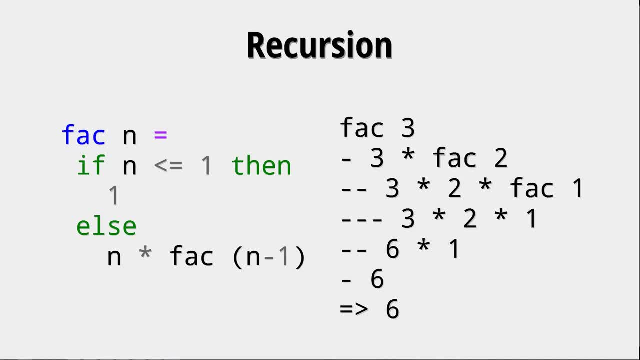 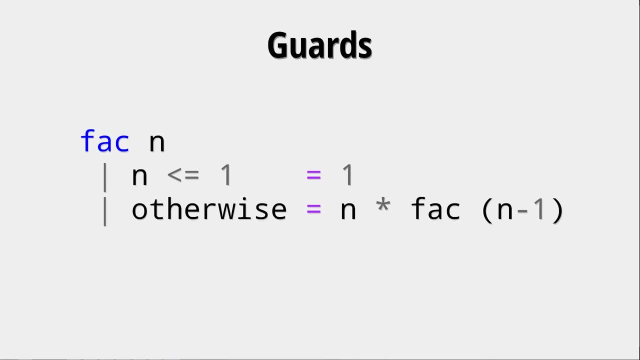 this is how you can recursively well compute the faculty, but also compute anything. It's very important to know that the faculty of n is n times the faculty of n minus one. There are different ways of writing this sort of if then else you don't have to use if then else. 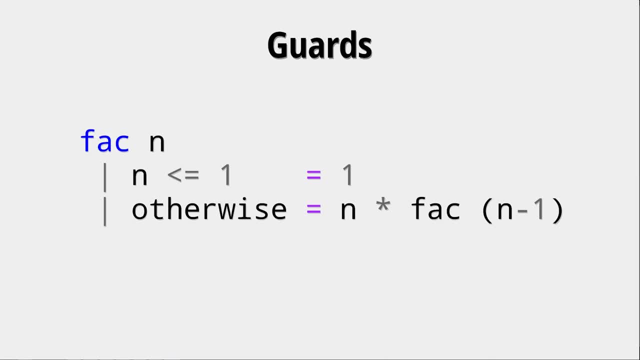 and it's important to understand that. if, then else is just another expression, But another way of writing. a function that has to have different functionality based on some Boolean expression can be done with guards. The good thing about guards is that you cannot just have two, but if you want three, four, five or any other finite number of guards, In this case 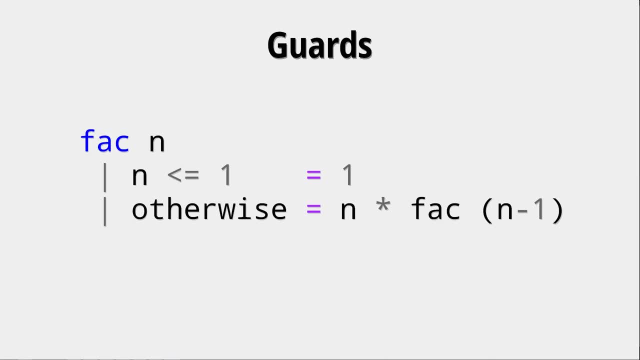 a guard has to have some boolean expression like n is smaller or equal to 1.. And the first boolean expression, the first guard which evaluates to true, will be the one taken as the definition for the function, for any function application. So we see here that we can just 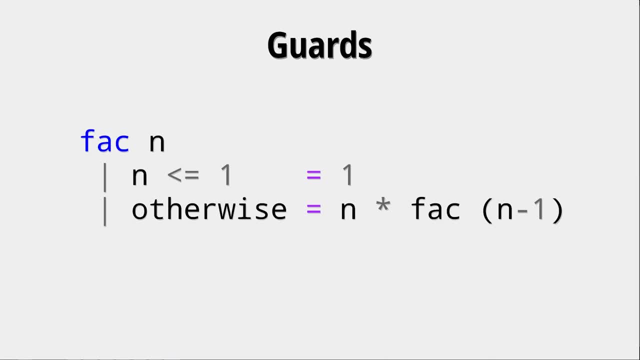 rewrite this, if then else as guards. Now it might be interesting to know what this otherwise is. This otherwise is just a constant which always evaluates to true. So that is why this last guard, this otherwise guard, is always taken, because it always evaluates to true. 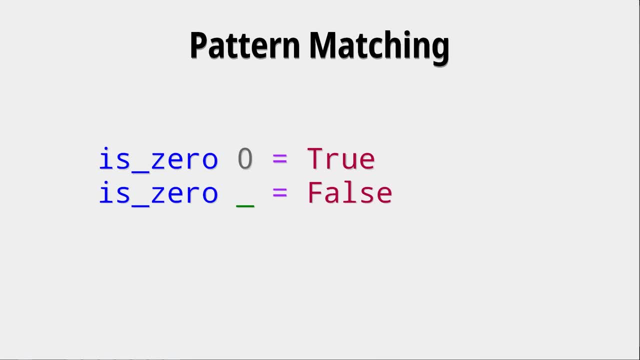 Another way of doing a very similar thing is pattern matching. Now for integers. pattern matching is not that interesting, like we can see here. What we're saying is that well is zero. of zero is true and otherwise- this other case- matching- is not that interesting like we can see here. What we're saying is that well is zero. 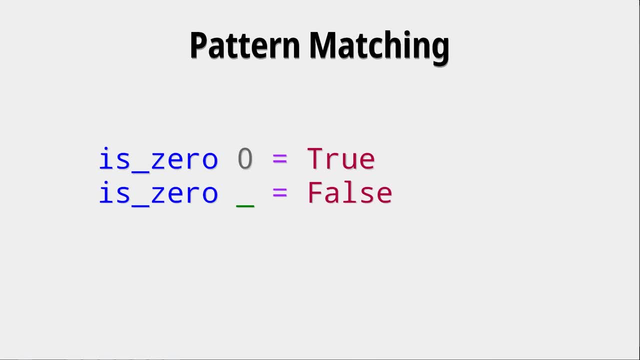 matches. So what does that mean? Well, we will look at pattern matching a bit more extensively in a later video, But here what you have to understand is that this underscore means we have a wildcard. This means that any pattern that can arise will match at this point. So here we have two. 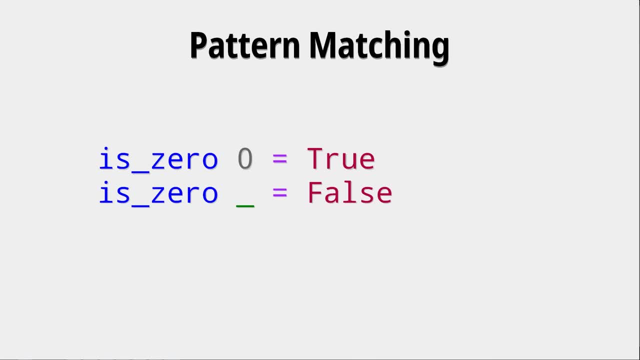 definitions of this is zero, just based on different patterns. In another language you might say: well, this is a duplicate function definition. We have two definitions of the function, But this isn't true in Haskell, Since the pattern of course makes this function partial, since is zero of zero only works for the value of zero, So we need this other definition. 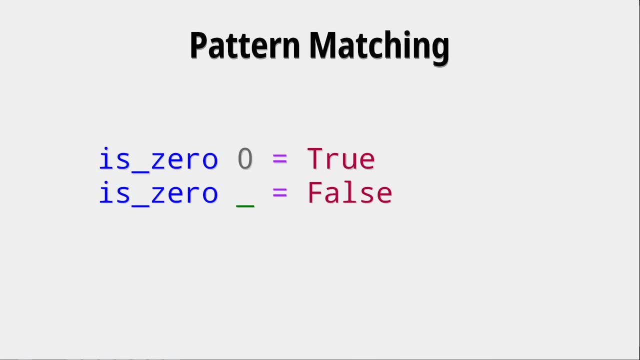 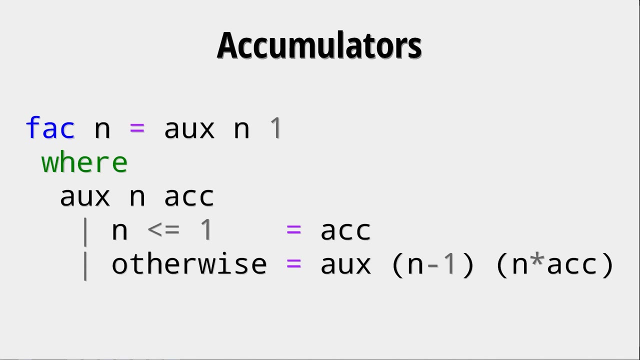 with the wildcard, where we can say: well, if the definition of is zero for zero doesn't work, for example because we called is zero of one, then this other definition holds. Another way of implementing recursive functions is with accumulators. Now, in this case we say that the faculty function is the result of an auxiliary function, aux. 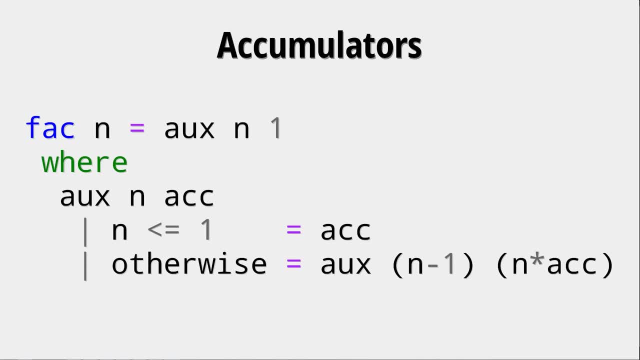 This auxiliary function takes another argument called acc or acc, which is our accumulator. Now, in an accumulator, you can, of course, accumulate some result, and that's what's being done here. So what we're saying is that, well, if n is smaller or equal to one, we do not return one. 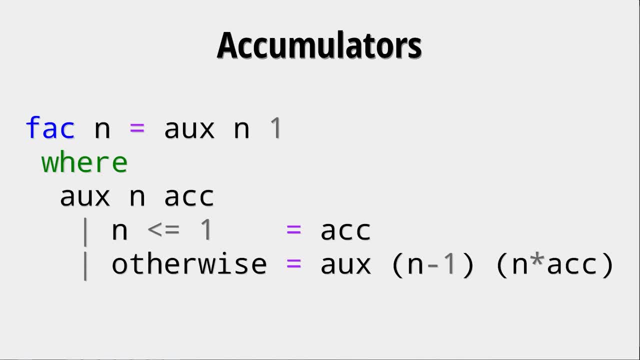 but the accumulator, Whatever. Our result at that point is. Otherwise, we of course update n with n minus one and then compute the intermediate result or the result we just get to that point by multiplying the accumulator we had with n. Now the question is: why would we do this and why is it helpful? 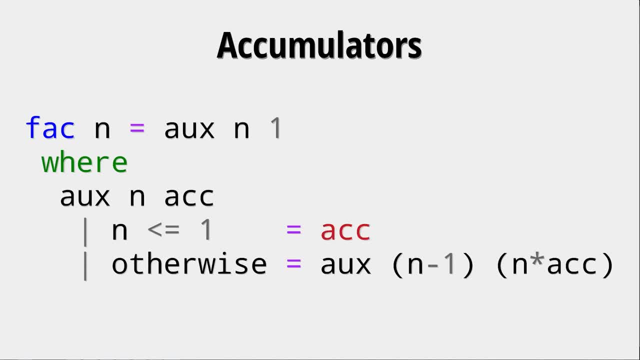 Well, let's look at what the definitions of this auxiliary function are. In the first case, we have a function aux. In the first case, n is smaller or equal to one. we return a constant. This is a constant. It at least is a constant value, since that is what our auxiliary function gets anyways. 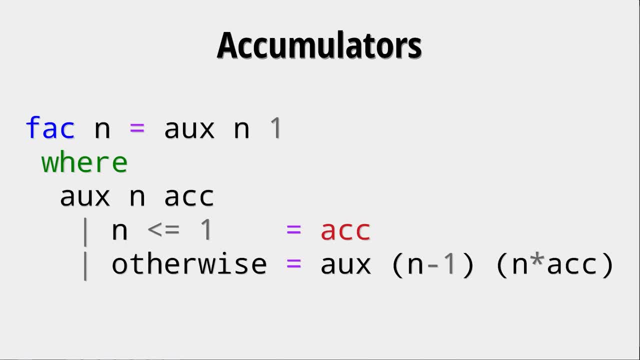 So this definition is no problem. We just return the value acc that we got in the function call. The other possibility is to do a direct recursive call where we have no operation after it. Think about how we defined the faculty function Before. we said that we take n and multiply it by whatever the result of the faculty n minus one is 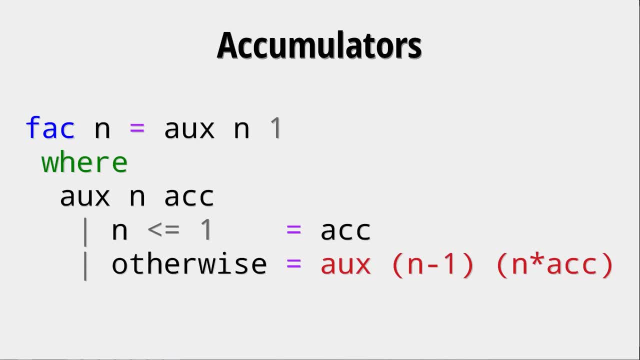 So we did the recursive call and then did a computation. That is not what we do here, because we compute n minus one and then we compute n times acc And we throw that into the recursive call. So this is what we call a tail recursive function. 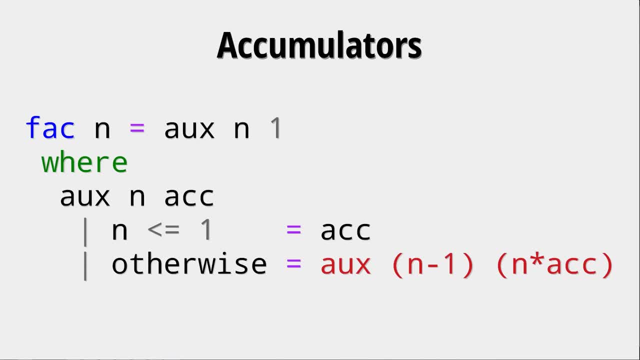 Since it has a tail recursive function, It has no operation after it's recursive call anymore. This is very important because clever compilers can basically rewrite such a function as an imperative function, For example with a while true loop. So in this case it does the recursion in quotes basically with a while true loop, and if we 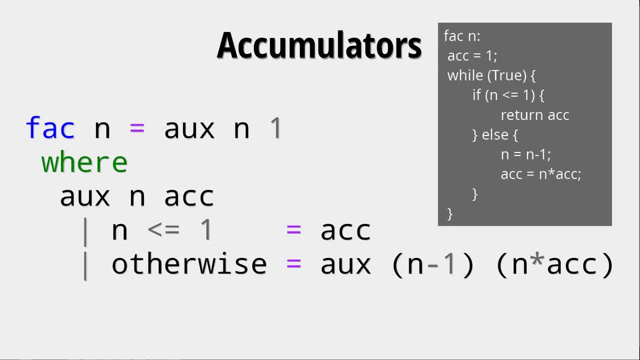 have the condition that n is smaller or equal to one, We can return the accumulator, and otherwise we update n and we update the accumulator and just continue. Because this is what we're essentially doing when we're using auxiliary functions without having any operation after the recursive call. 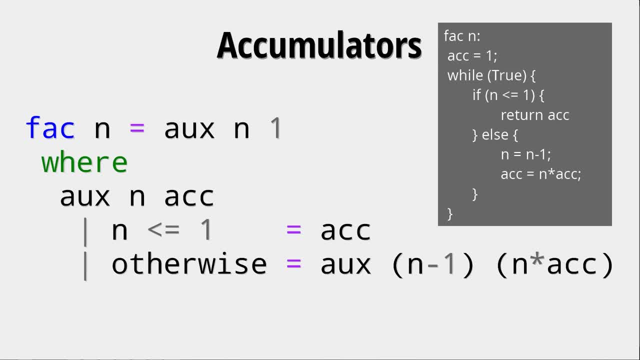 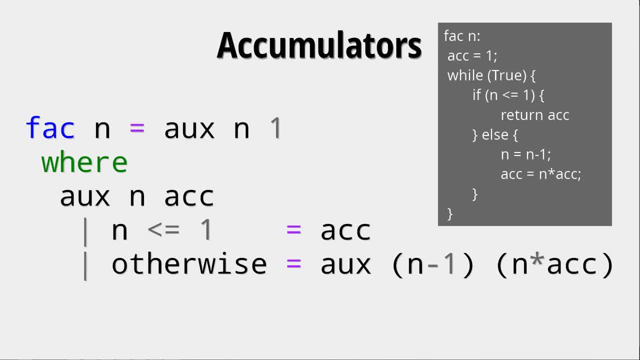 Now, the stack only has finite amount of memory, So the amount of recursive loops you can do is finite. Now, this is not something we want, because sometimes we want to have an algorithm that actually can loop to infinity if it wants, Like we do here, because we do not want our faculty function to be bounded by the size. 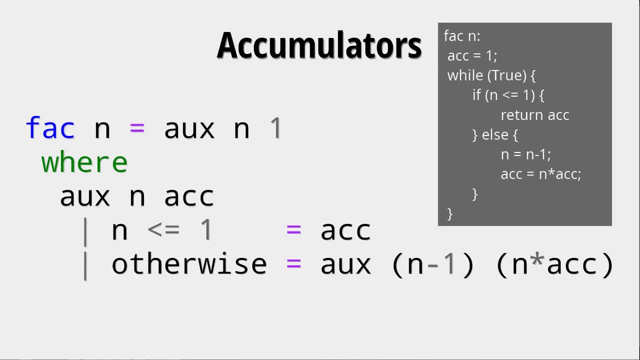 of our stack. Now this implementation. This implementation wouldn't be bounded by our stack, because a clever compiler can optimize this function to be imperative, where we don't even need a stack anymore, because we call the function only once and then we end up in this wild, true loop.